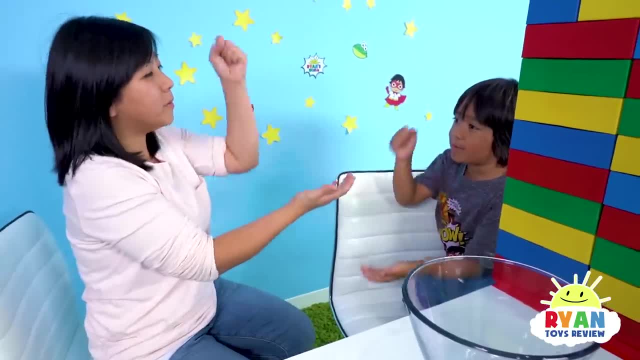 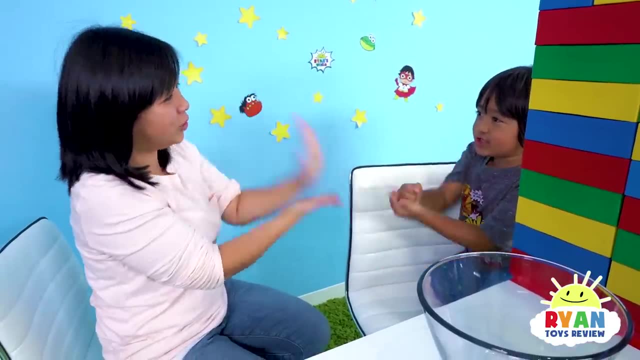 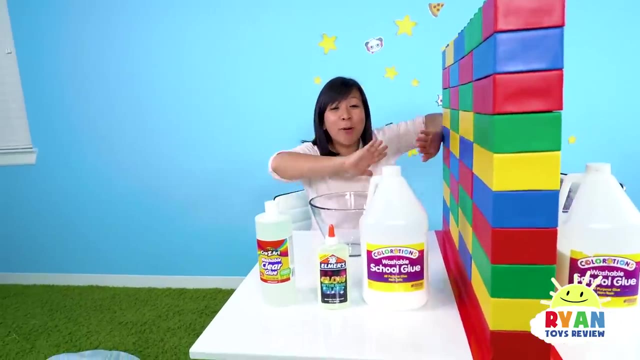 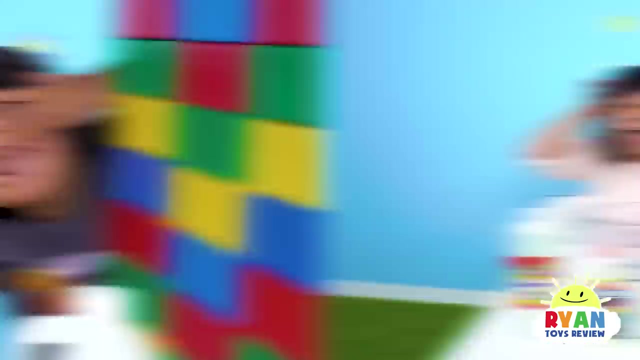 Is that a hint? No rock paper scissors shoot tie. rock paper scissors shoot. rock paper scissors shoot Right. so I get to choose: and no peeking Ryan, no peeking. Okay. no peeking Ryan, I'm closing my eyes. No, you're not Ryan, look at him, He's not even closing his eyes. I'm gonna go with. 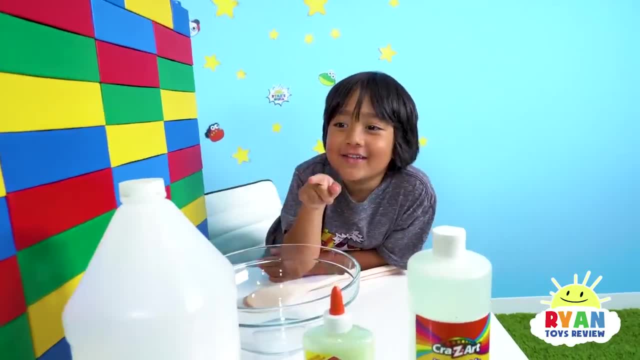 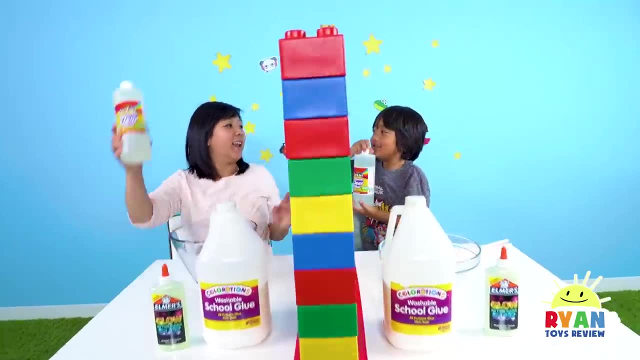 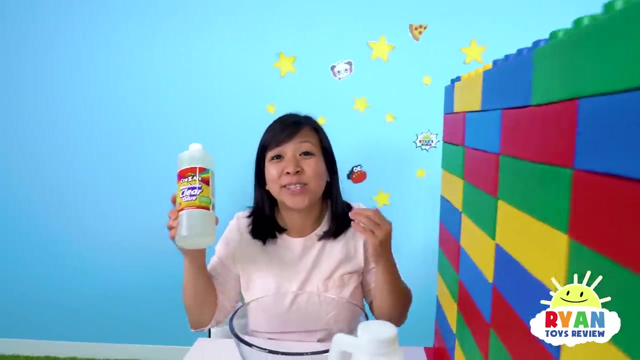 Okay, all right, Ryan, your turn. hmm, I really like this one, but I have a feeling mommy's not doing that one. This one, three, two, one, What? how? How did Ryan guess correctly? Yes, two points, two points. Whoa. so Ryan guessed it right, so he has two points. I'm gonna do half. 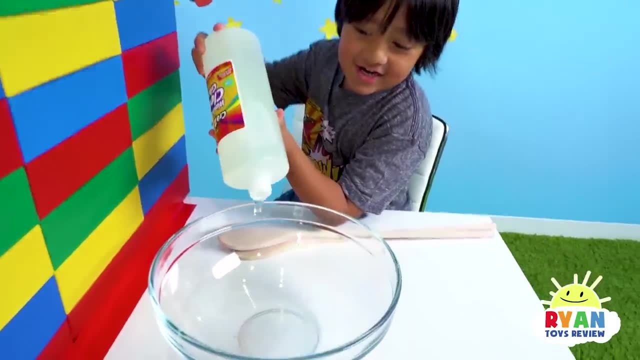 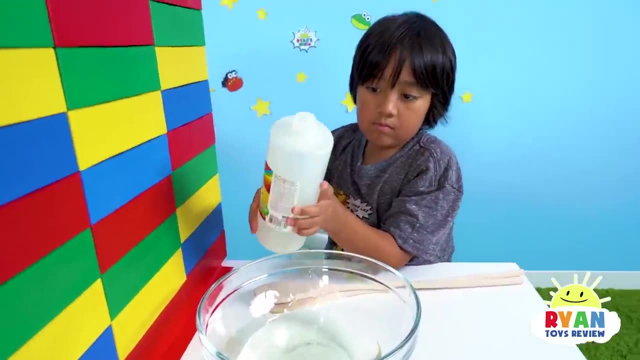 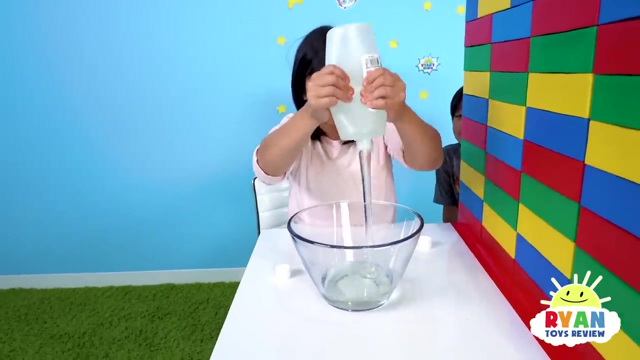 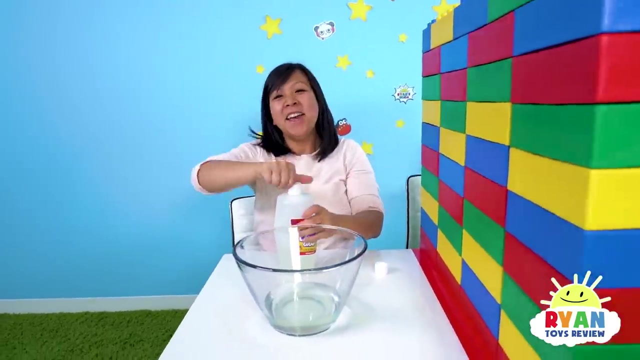 me. This is the glue three, two, one. I also picked the clear glue, so We'll be cool if it's clear slime. How do you do that? I don't know. I'm strong. He got some mommy muscles All right. next round, do a little bit more. now we're doing which color glue we want. 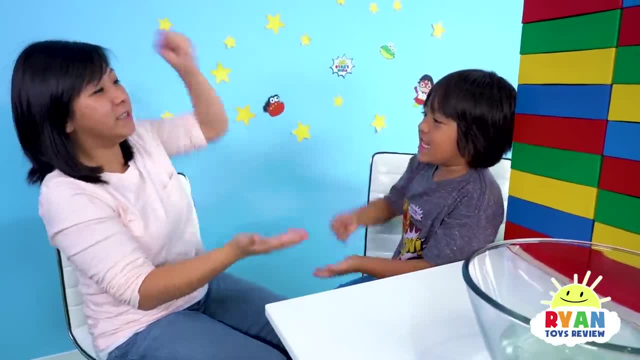 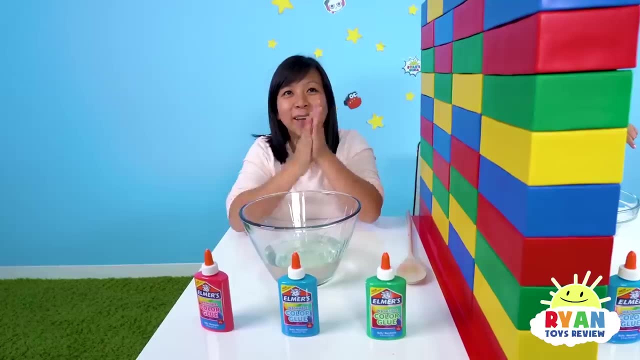 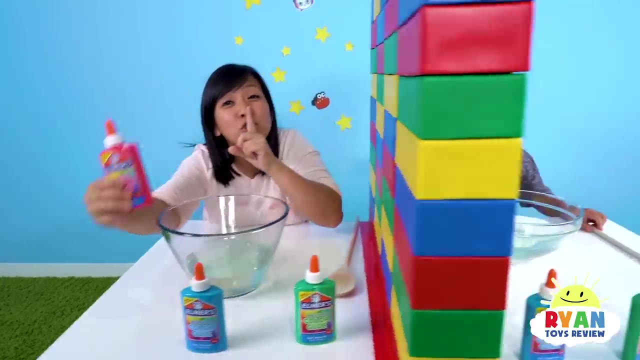 red, green and blue rock paper scissors shoot No peeking, no peeking. I'm not for realsies. What color will I choose? I love all these colors. You don't want to pick here. You know I can barely hear you right. so what? we said something's wrong with the ass. 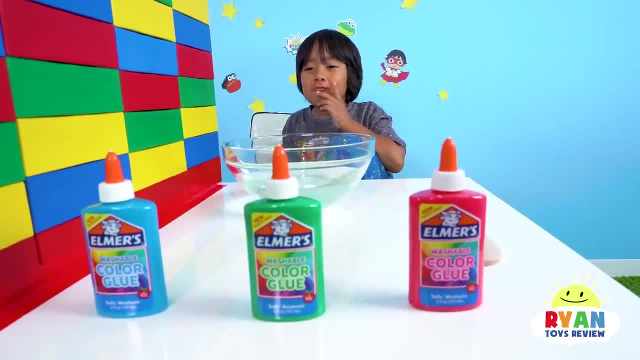 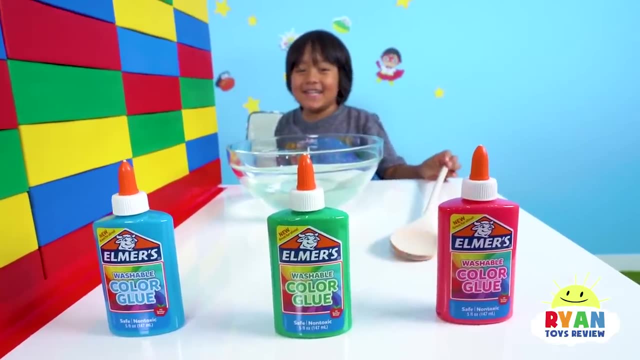 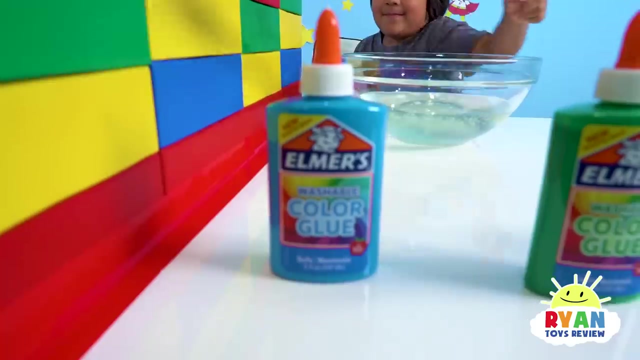 No grass. no grass is not starting with an S. You ready? Yeah, this glue. right, you make this look complicated. you've got color, What is it? Let's do it together on the count of three ready, one, two, three. I picked this glue. 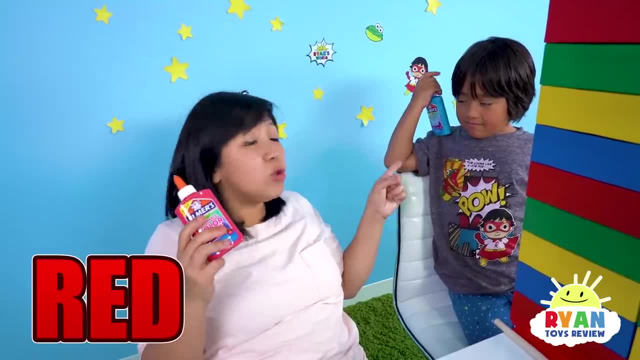 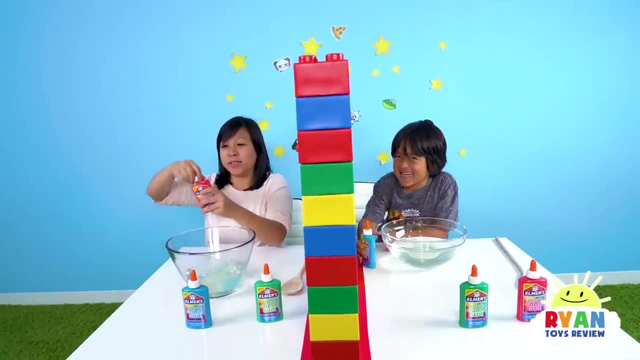 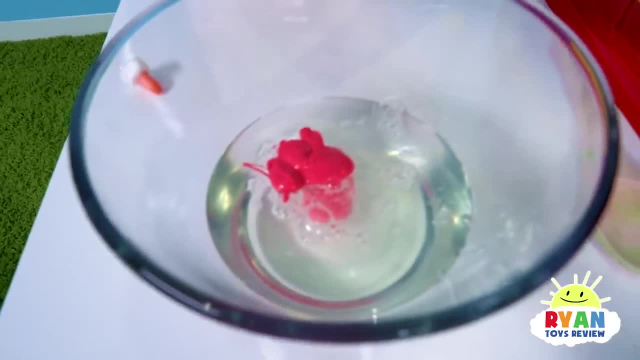 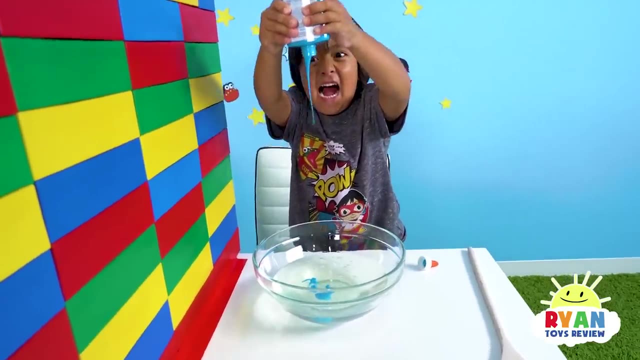 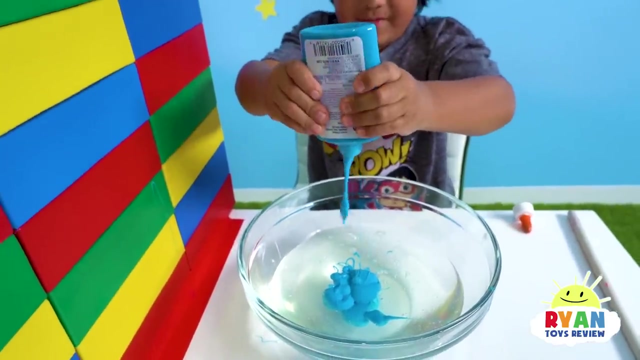 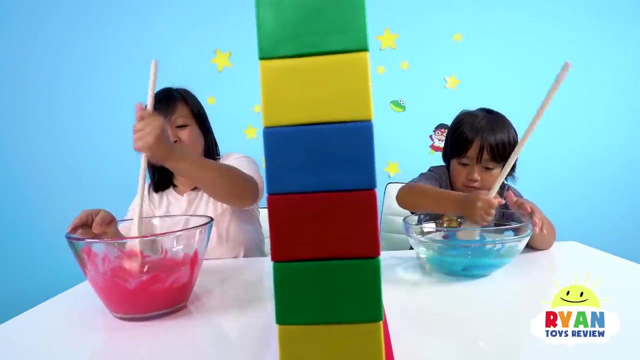 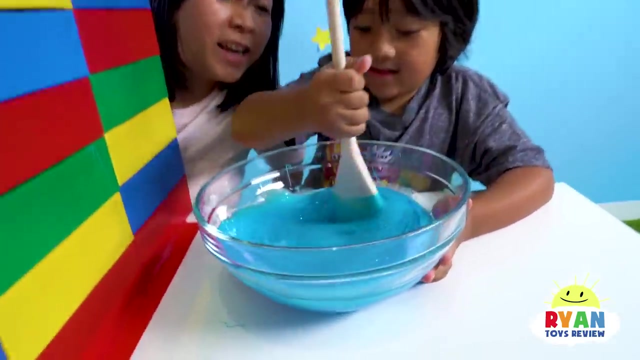 Go red. Mine makes like a pig noise now let's mix it. So much for clear. now is just like pinkish red mommy. look at mine. Oh, it does look quite like yours, Ryan. I think yours looks prettier than mine. We see yours. 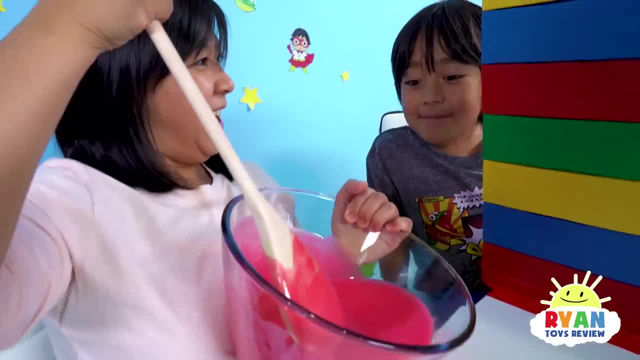 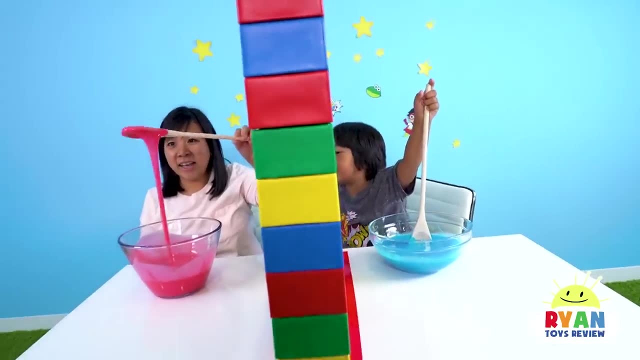 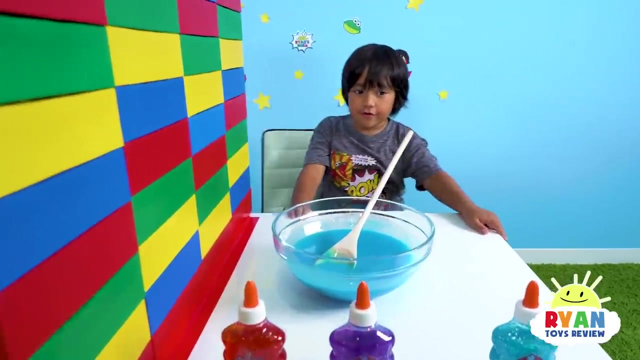 Wow, yours looks like Maybe a pie a pie, Or maybe you burn apples, so then it looks like a caramel. Yeah, Oh, Okay, gotcha next round. now We're doing the glitter glue. We got blue, which I'm not gonna probably do blue, because I already have blue. 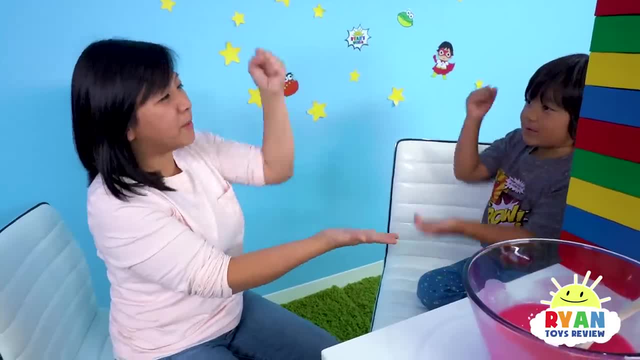 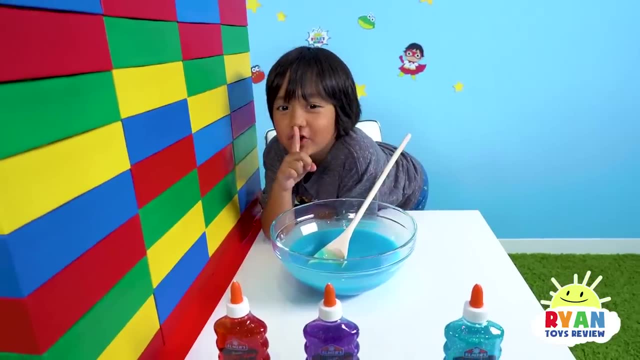 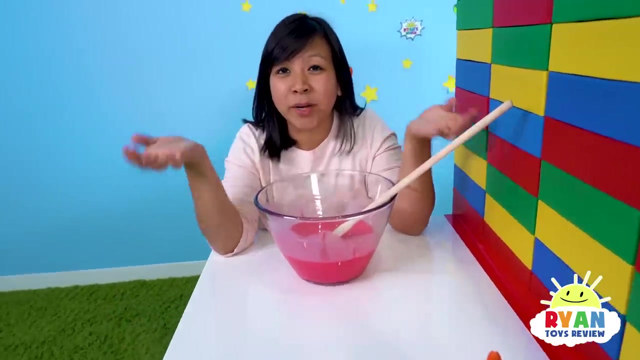 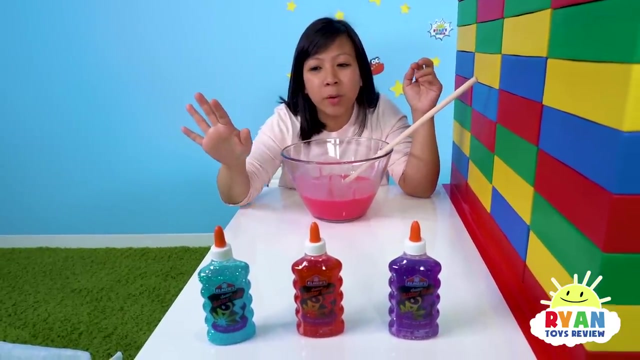 And I'm purple and red rock paper scissors shoot. Oh, You got it. Okay, right, I'll let you decide then. Oh, Hmm, this one Ryan, says he's not gonna pick blue because he has already have blue. But what if he's just tricking me and pick blue, right, Am I right? I don't know. No, I don't know. Okay, so I'm going to pick. 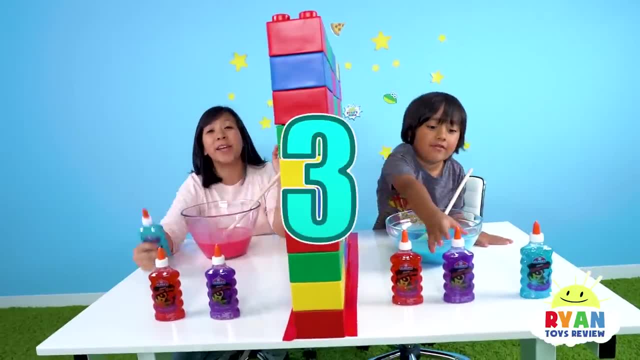 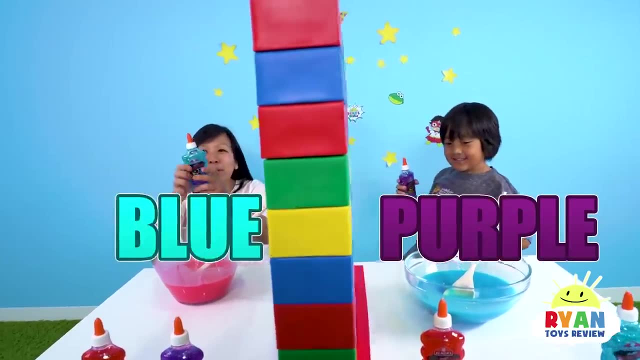 Are you ready? I got a three, One, two, three. Did I get it right? I was not lying. So Ryan picked purple and I picked blue. so I didn't get a point and Ryan got a point. So that means Ryan's three points and I have one. 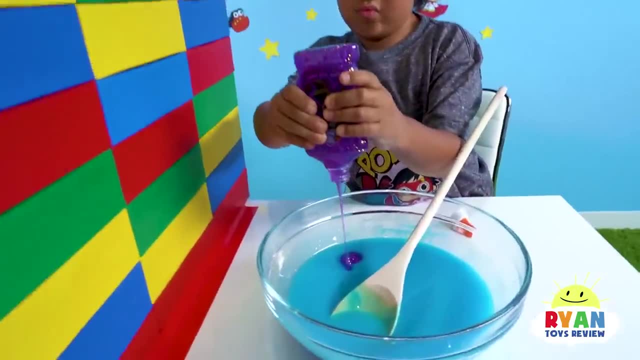 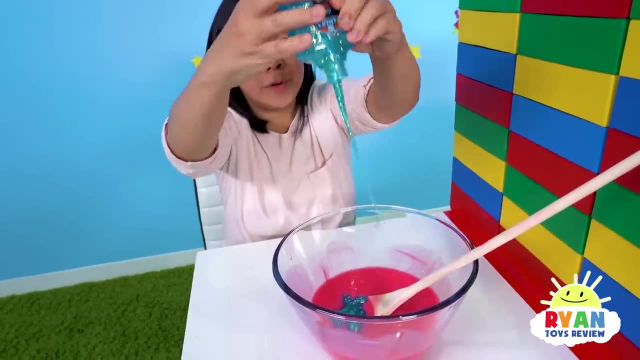 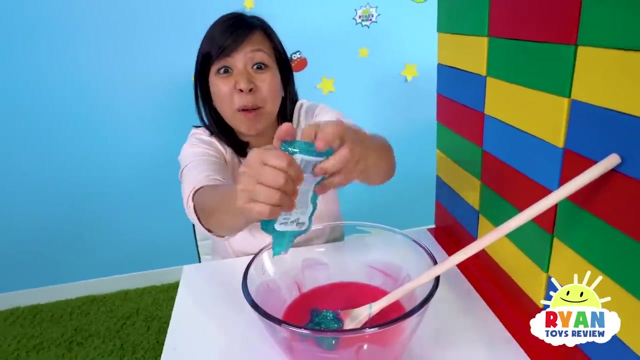 Three, two, one. Oh no, mommy, I think I'm gonna have like dark purple and dark blue. my Blue is so pretty, but I think I'm gonna have purple too, Ryan, actually, because blue and red makes purple. Oh, Oh no, mommy, What I have too much blue. Oh, it's okay, So you won't even see it. 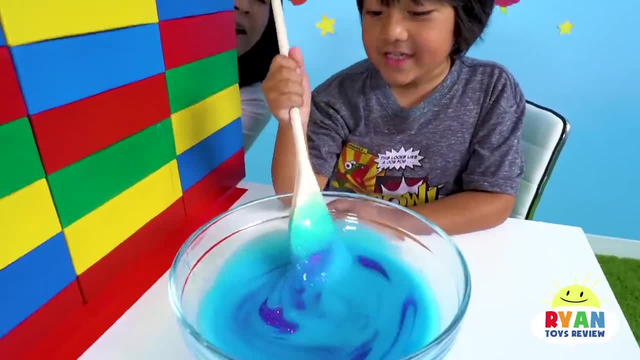 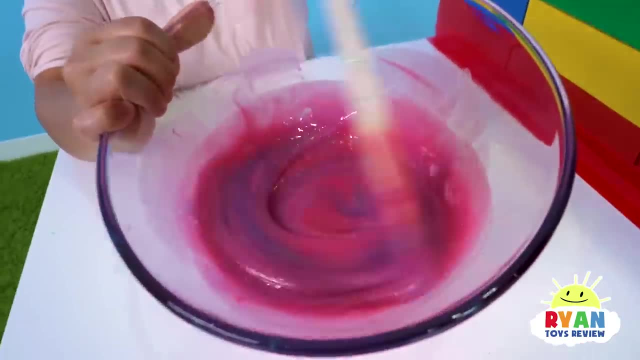 It's gonna just disappear. No, it's going to look like waves. Oh, maybe you just have glitter. Mine looks kind of cool. Oh, I lied, it just makes my color more dark. I don't like it. Yeah, I liked it better before. 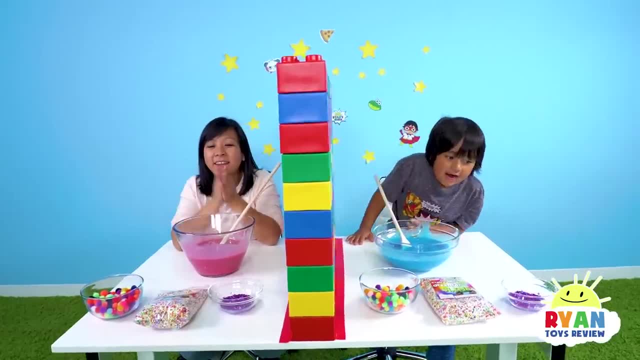 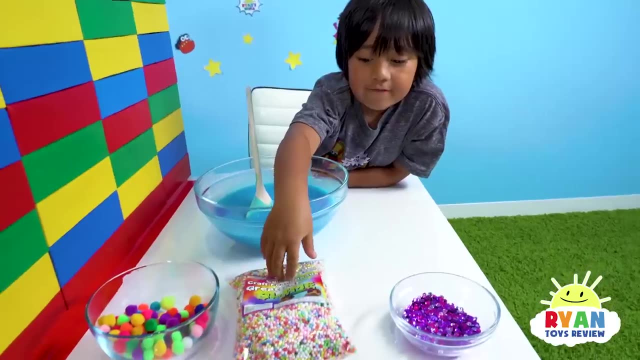 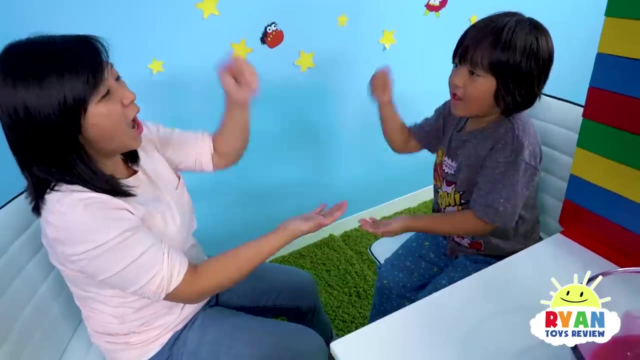 okay, guys, next round. Now we have some blue, some glitter. i actually love these. it might not be a clue. it might be a clue. we have some foam beans and some fluffy balls. oh no, raw paper scissors shoot, oh no. so ryan beat me, so he gets to decide. 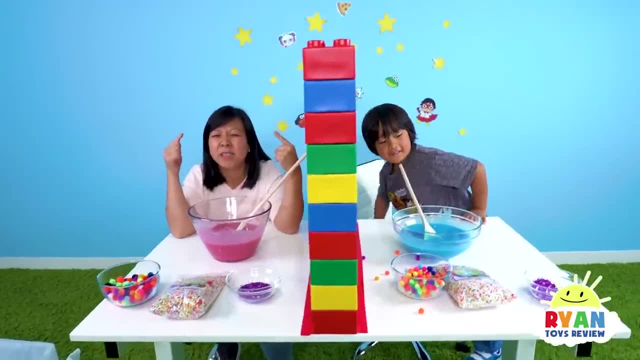 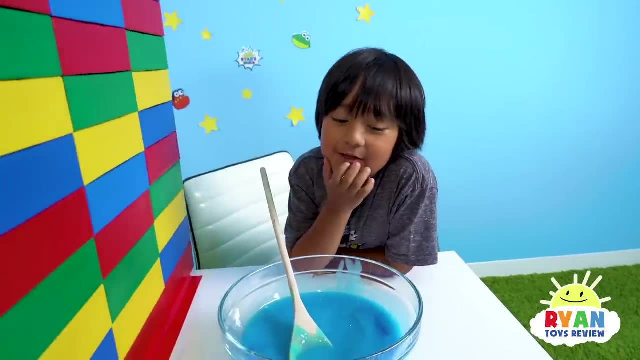 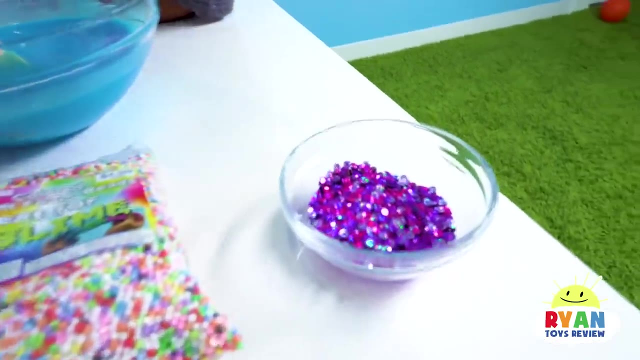 which one. this is tough. go ahead and decide. i'm gonna just try to think. i love the purple so much, but i think mommy's gonna pick it. i'm probably not gonna pick purple. i mean the glitter- is that yours? yet i don't know which one i will pick. i'm gonna think ryan's going to pick. 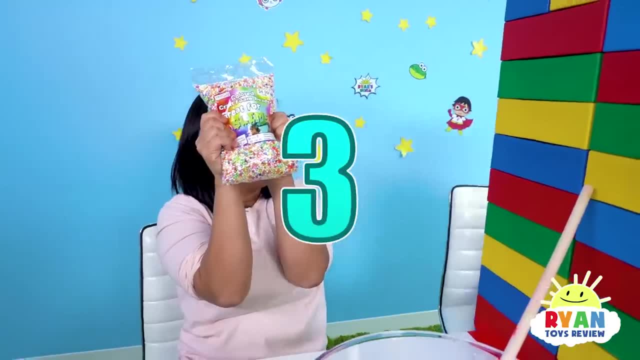 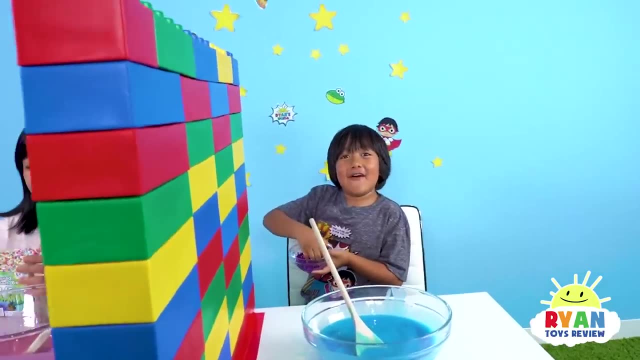 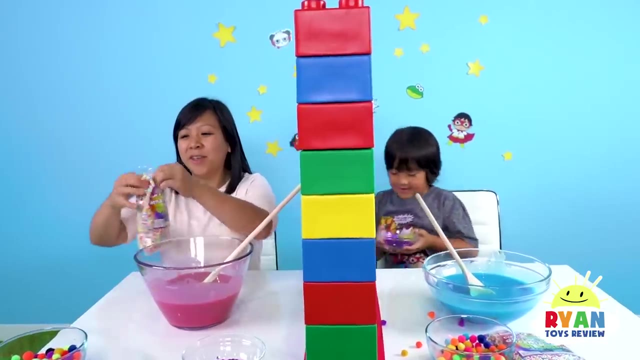 this one because it says great for slime. did i pick right? three, two, one? i didn't pick right, mommy didn't win, so i got four points and mommy with one. i only have one. i need to catch up. all right, ryan, you ready to put in our little fun accessories? yeah, three, two. 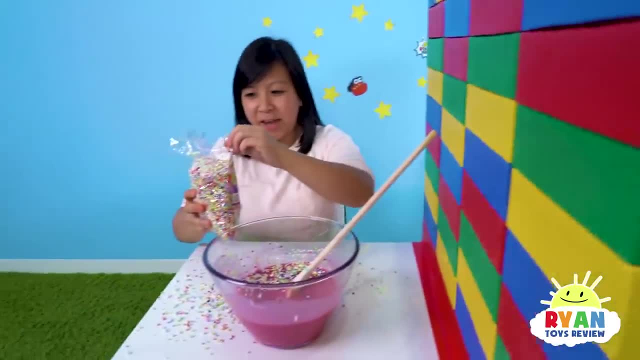 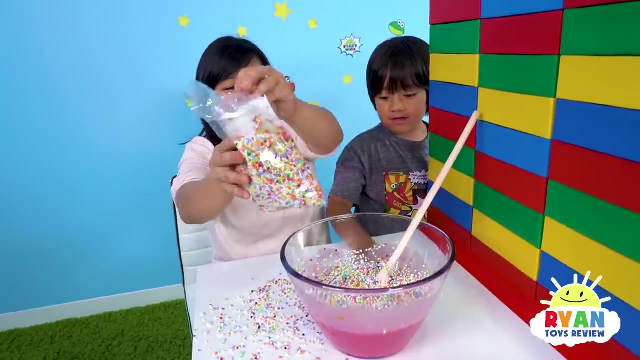 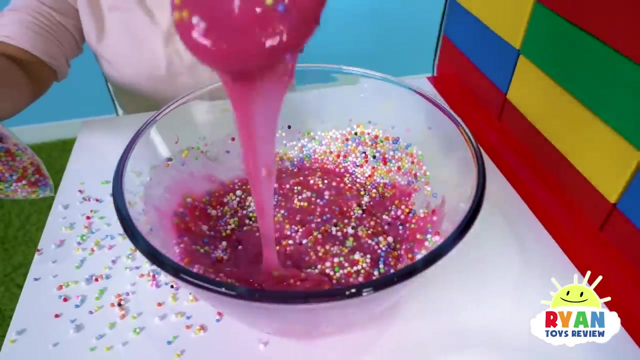 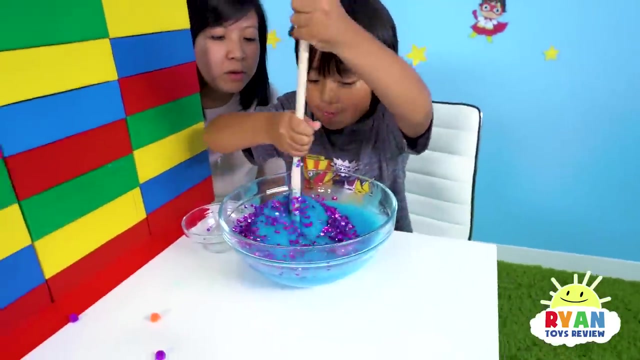 one, so i accidentally spilled it everywhere. you're gonna get two pieces. okay, that's enough. all right, i'm gonna just mix it up here more. oh, this looks so funny. what'd you guys think? yeah, how's your looking right? oh no, i'm burying mine. don't marry, you, don't bury. please don't bury guys. 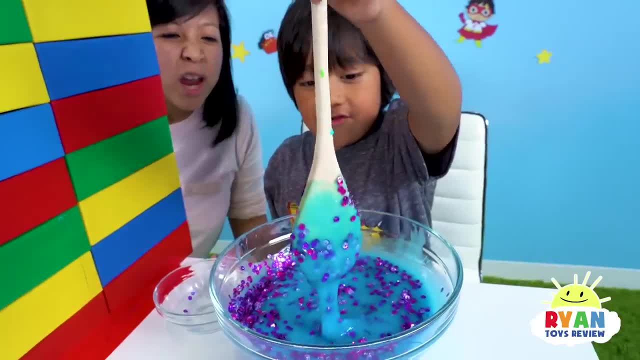 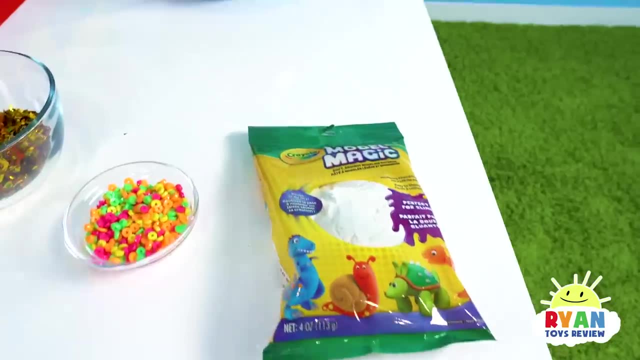 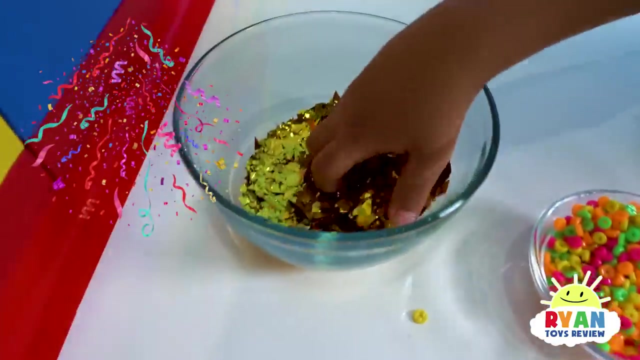 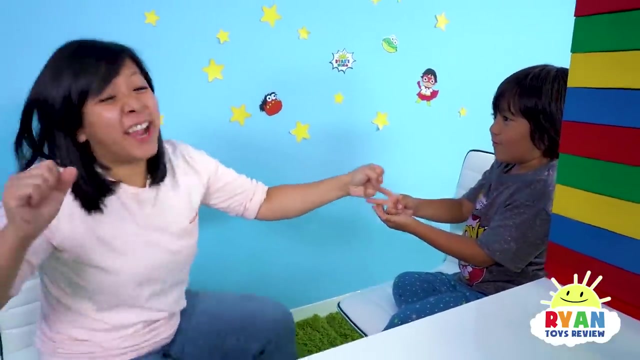 yours looks awesome. all right, we're gonna keep mixing and wait for the next round. now we got some like play-doh stuff and says: perfect for slime. and we got some beads and some confetti. are you ready for paper scissors? yes, rock paper scissors. your shoe. i follow me. ryan, i get to choose this time. okay, ryan, no peeky, i get to decide. 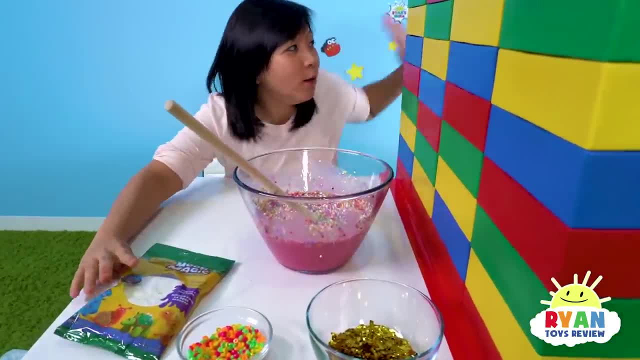 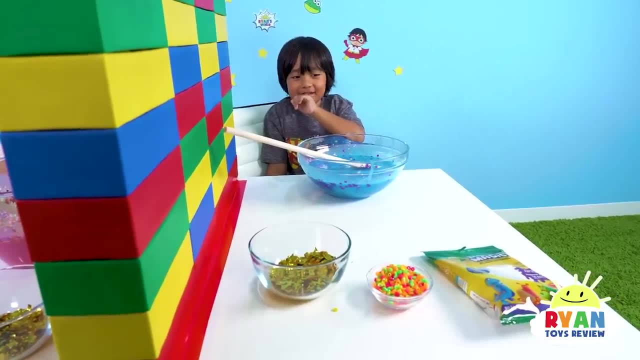 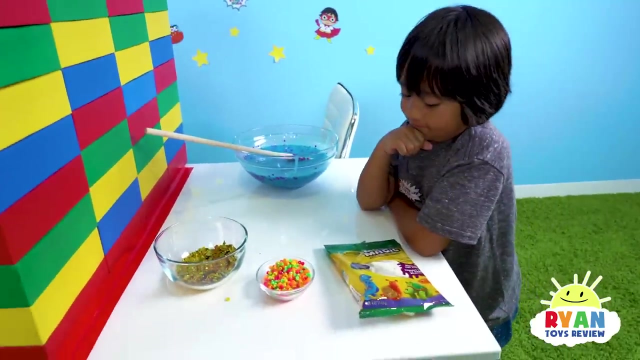 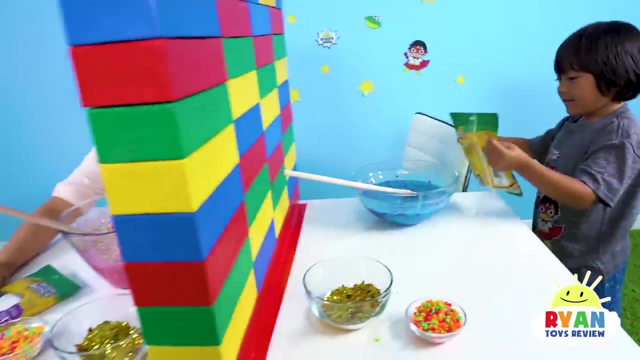 they all look really cool, but no, looking. okay, ryan, go ahead. i heard, why are you making sound? i'm not, i'm not, i'm just making radon sound. here go, ryan. which one got it for slime? okay, ready. one, two, three, this one. oh, we chose the same. that means ryan got it right, so he gets. 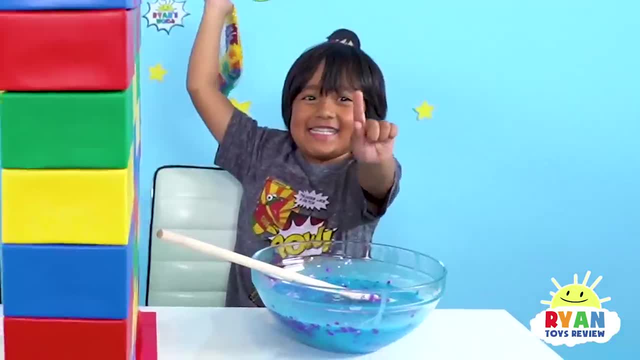 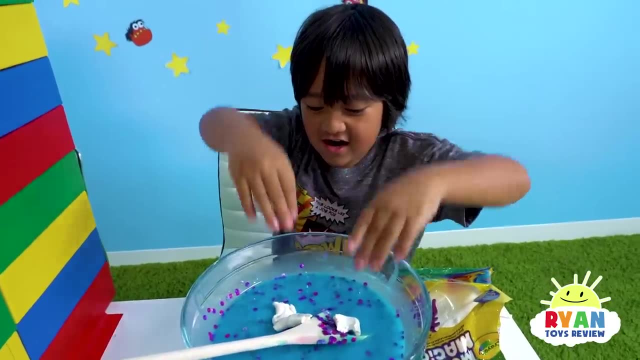 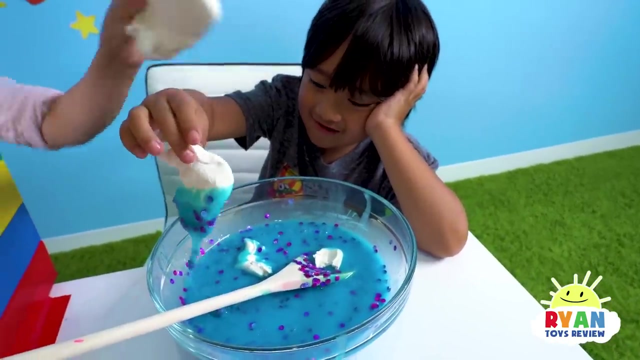 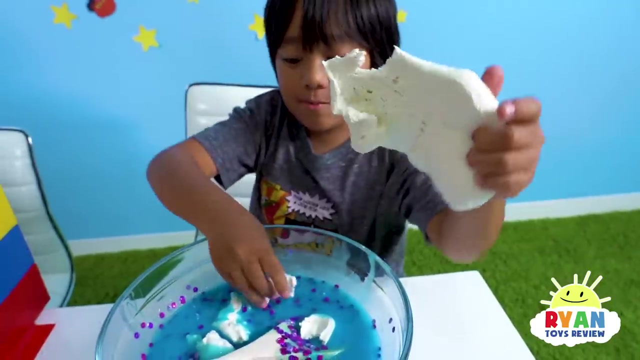 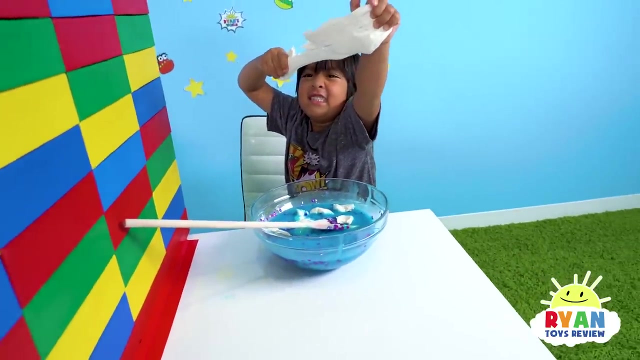 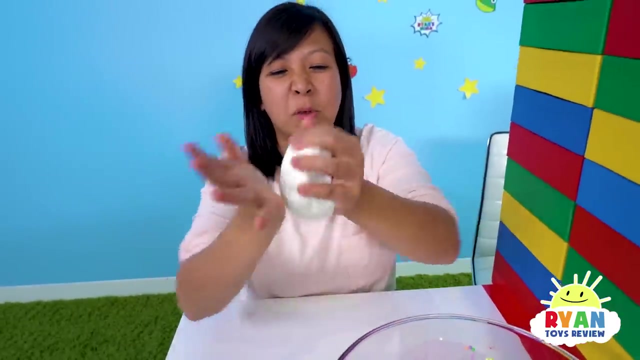 a point. i got five points, mommy got one. i only have one, ryan. keep getting it right. good job, ryan. that doesn't look good. it looks like a marshmallow, it does. you're right, gonna get a little pieces. yeah, yeah, my turn. look at this. i'm just gonna roll my up into a ball here and just dump the whole thing in. 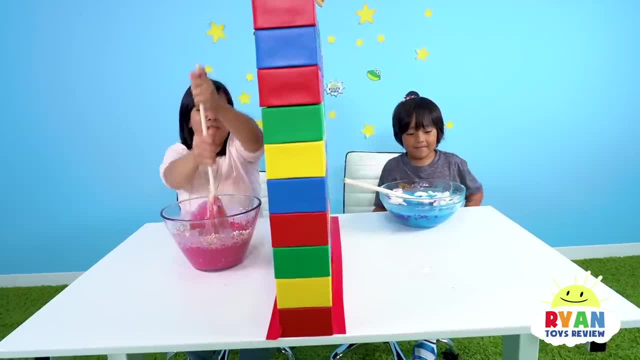 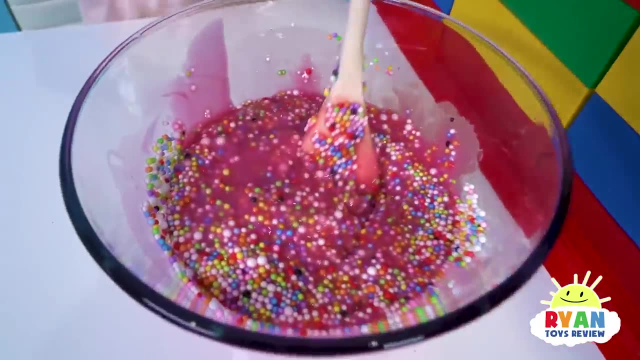 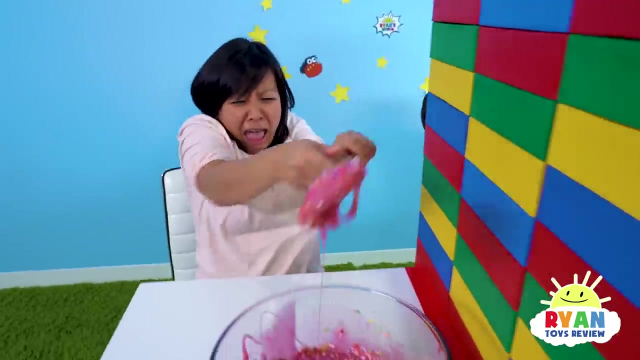 you ready: one, two, three. now we have to just smash it. we can't even like, mix it up, we have to smash it first. look, there's still like a big clump here, ryan, it's still there, mommy, mommy, you know why? it's because, mommy, it's because you put everything. 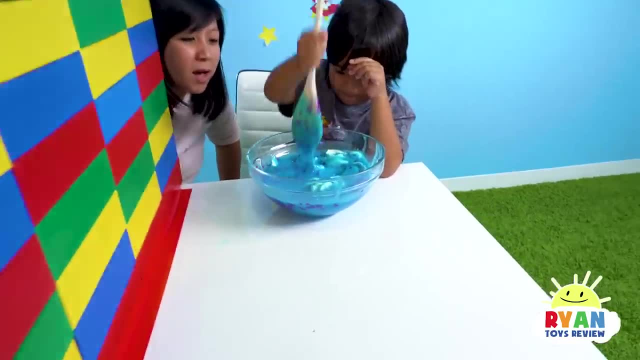 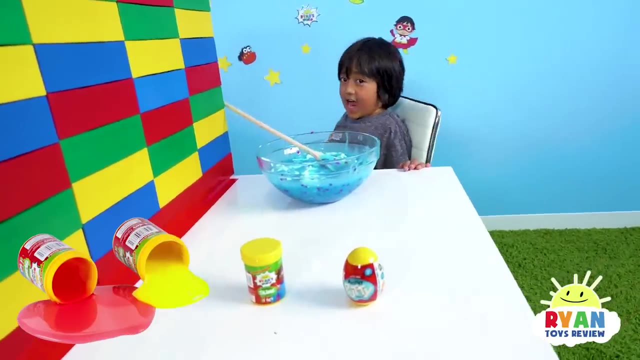 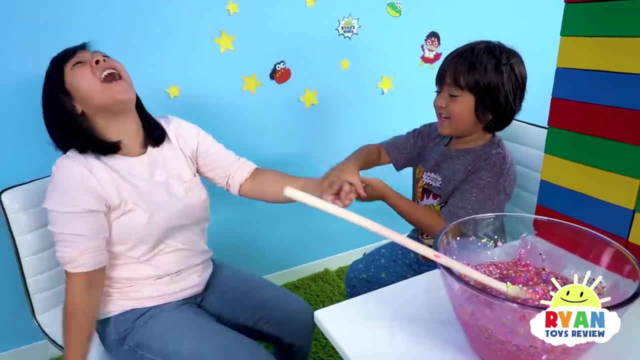 together. oh, yours is good, you smash yours up, very cool. all right, ryan, next round. now we're gonna do ryan's slime, ryan's putty, let's do rock paper scissors, rock paper scissors, shoot. oh, ryan won. okay, so he gets to decide between the mystery slime or mystery putty. 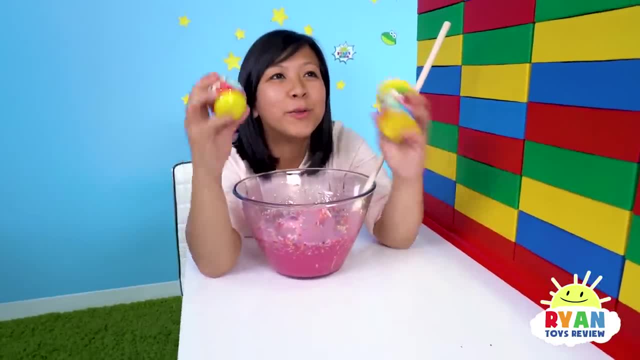 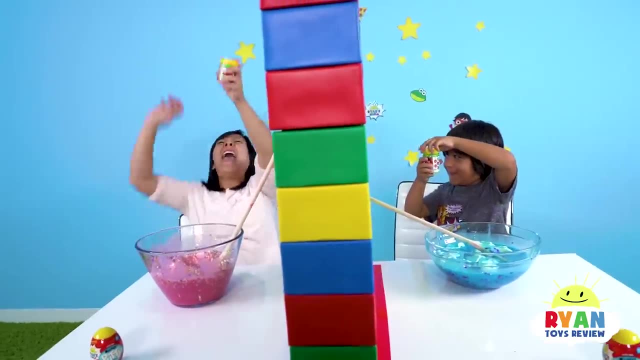 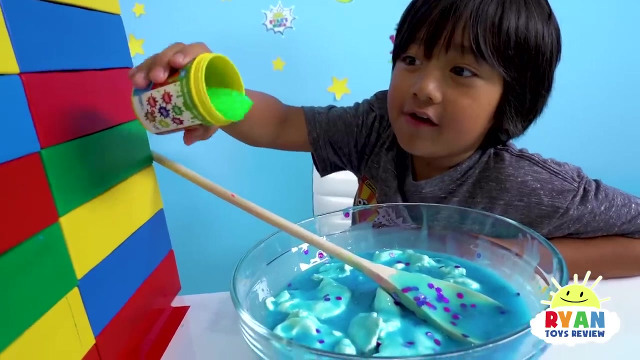 it's so hard to choose. i love them both, but since we're doing the slime challenge, so i'm thinking ryan will pick the mystery. did i get it right? did you pick the slime? yeah, i got a point. i have two points now. i got green, you got green, i'm gonna put it down. now i'm gonna put. no, i'm gonna pull. 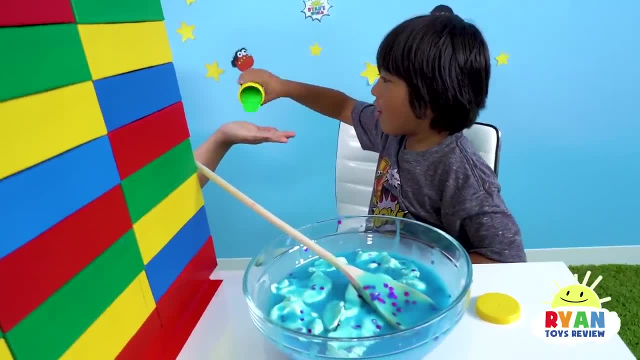 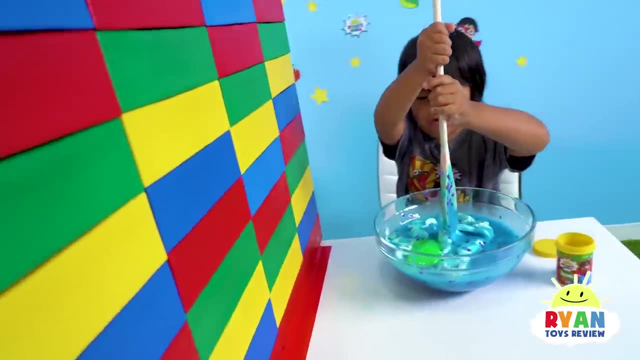 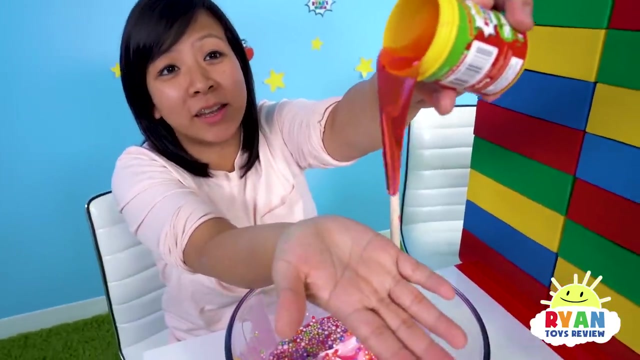 mommy, i'm gonna put it down. look, okay, whoa, you're a trickster. oh, very cool, ryan. no, now i have to destroy this one. destroy your smash. this is the color that i got. it is so pretty. look at this color. look how pretty this slime is. i love this color. 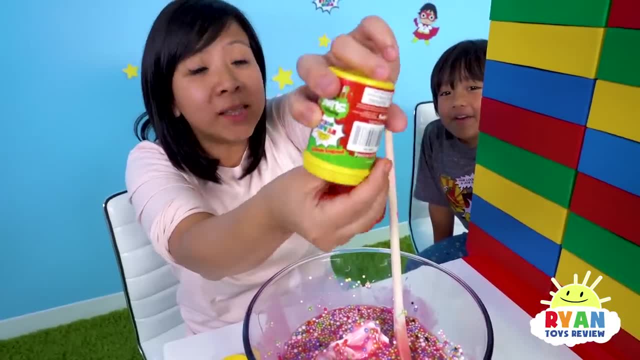 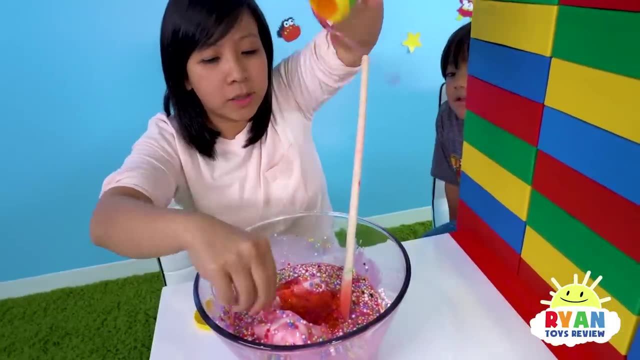 and it's perfect, mommy. pretty much nothing's gonna happen. yeah, it's perfect actually, because it goes with my color slime. so look at this like it's gonna just blend in really really well. so i have like this really cool pink color. mommy, remember, you actually can't break the slime. okay, so i'm gonna just 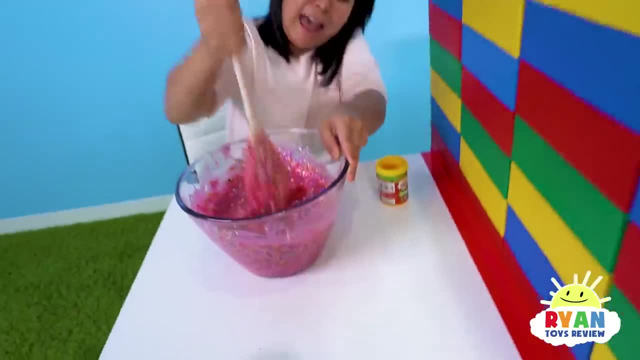 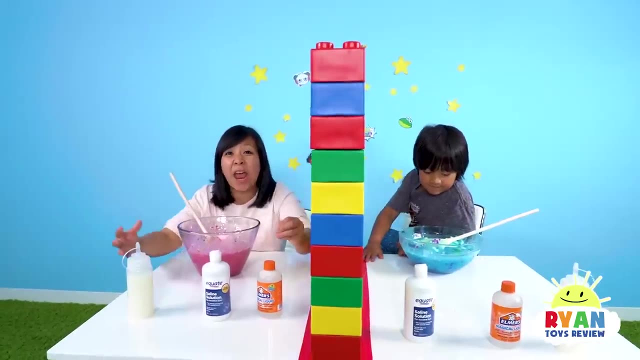 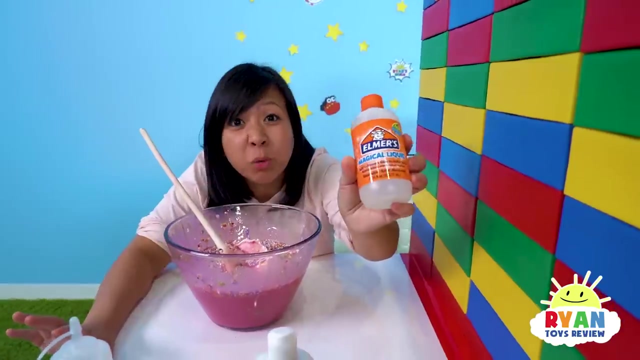 agitate and mix it up here. the clay still needs breaking. next round, last round: the secret ingredient to make slime, the activator. so we got three. we got some magical liquid here- okay, that's gonna make the slime. or we got some contact solution, or we got 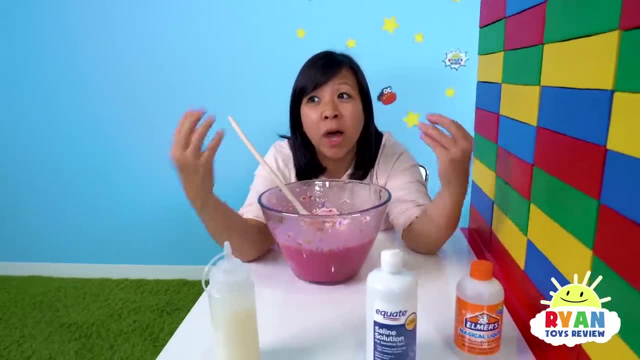 some liquid starch, okay, so let's look at this one. we got some magic hydra, and then in this one we got- Let's see what we picked to make the slime. Are you ready? Paper rock scissors, Rock paper scissors- shoot. 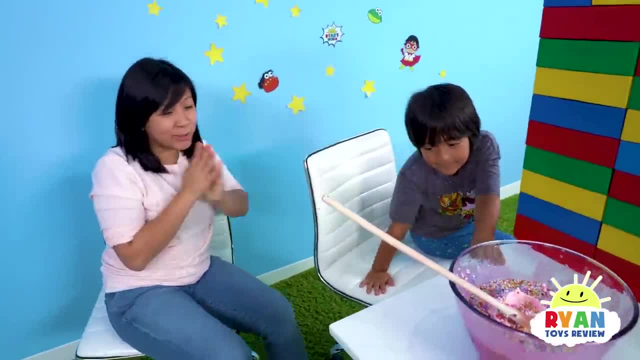 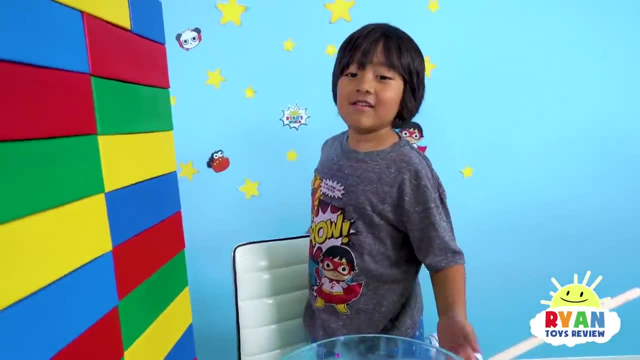 Ah-ha, I got, I cut Ryan, so I get to choose which one. I'm going to choose this one, Ryan, are you looking? Did you look? No, Okay, then you pick. then Which one are you going to pick? 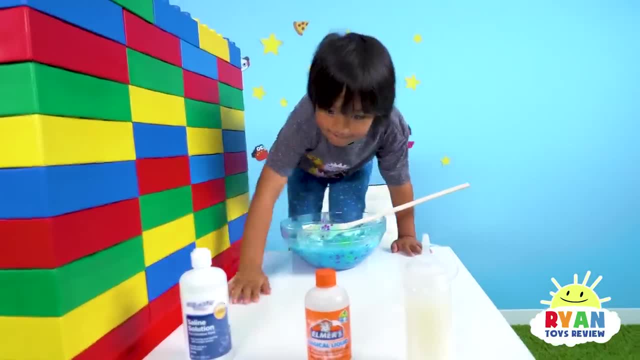 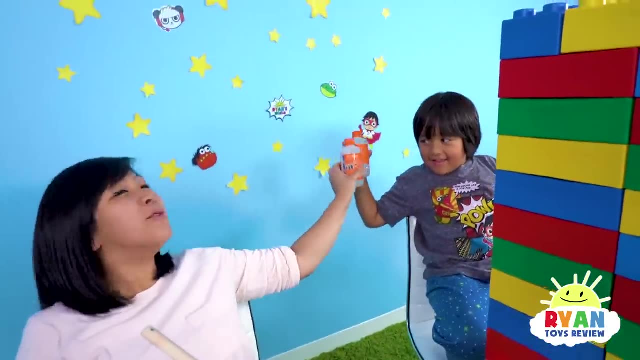 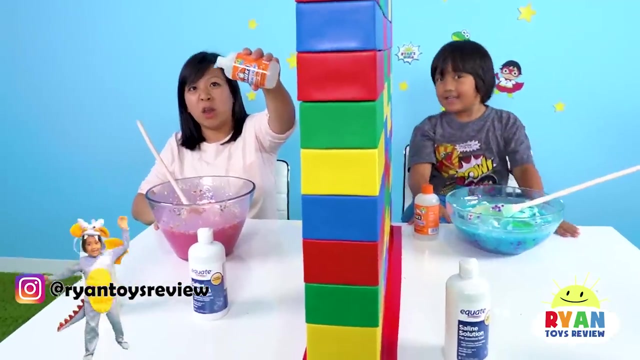 Shhh, Three, two, one, Wah-ha, same Wait. that means Ryan gets a point, Ryan with six points and Mommy has two. Let's put in our magical liquid Wah. Hopefully this will make the slime. 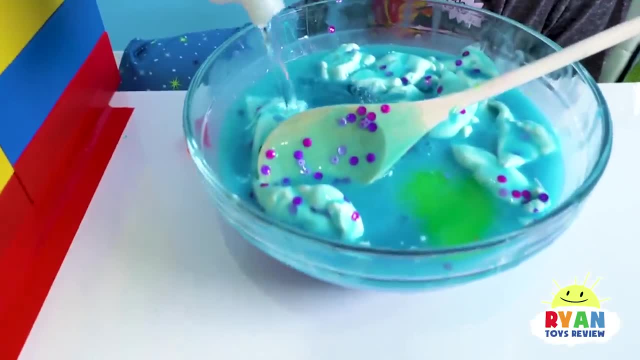 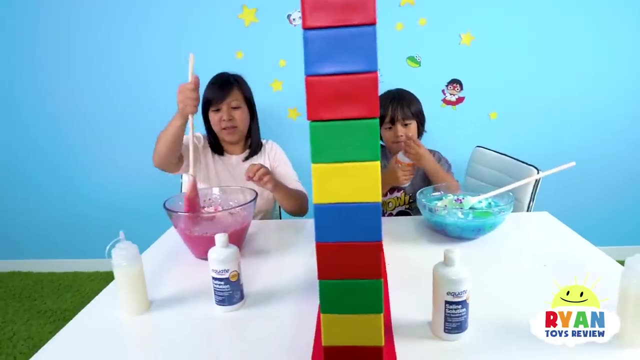 Yep, we got it. I'm putting it on an island. It's more safe if you put it on an island- An island, I'm talking about the clay. Now, once it's in, we just have to just keep mixing until we get our slime.